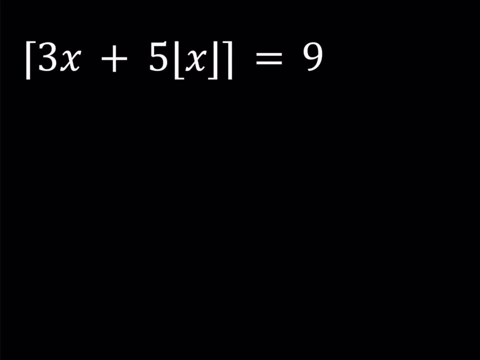 Hello everyone. In this video we're going to be solving a floor and ceiling equation. So we're given that the ceiling value of 3x plus 5 times the floor value of x is equal to 9, and we're supposed to solve for x values. Let's go ahead and quickly remember what those values. 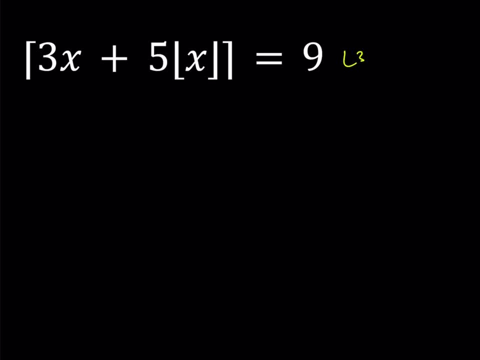 are. If you have a number like, let's say, 3.14, and you're trying to find the floor value, it is going to be 3 because you're supposed to round it down to the nearest integer. And if you have the ceiling value of an expression or a number, then you're supposed to round it up. 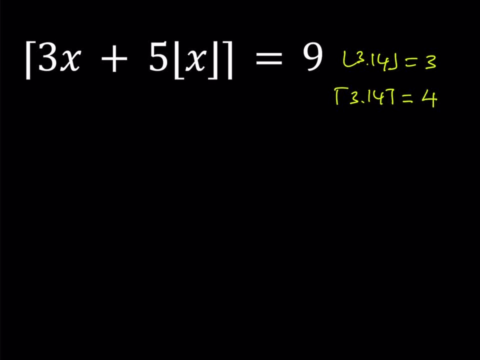 to the nearest integer. In this case it will be f4.. Now let's go ahead and start by naming this floor value of x: n. So I'm going to name this n, and this gives me floor value of x equals n. 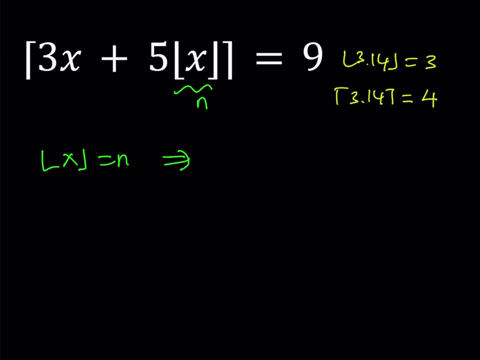 and obviously this gives me an inequality. So one of the nicest things about floor and ceiling equations is that you start with an equation and then you get an inequality and then you solve it and then you get an equation, so on and so forth. So you kind of go back and forth. 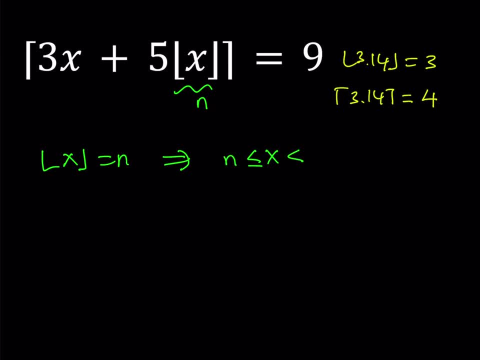 This implies that x is between n and n plus 1.. So x is greater than or equal to n and at the same time less than n plus 1.. The second one comes from our equation. when we do the substitution, 3x plus 5n is equal to 9, and this implies that 3x plus 5n. now you got to. 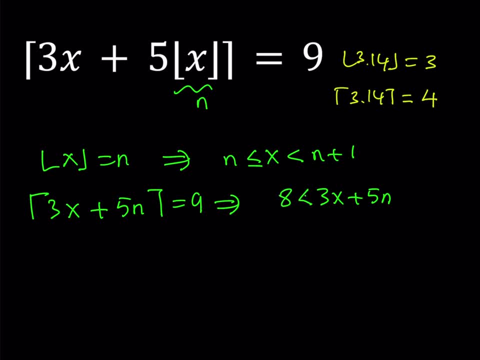 remember, this is the ceiling value, so we can take anything greater than 8, like 8.2, 1, but it also needs to be less than or equal to 9.. If you have an integer, its floor and ceiling value are going to equal the same integer. Okay, now we do have two inequalities. Let's go ahead. 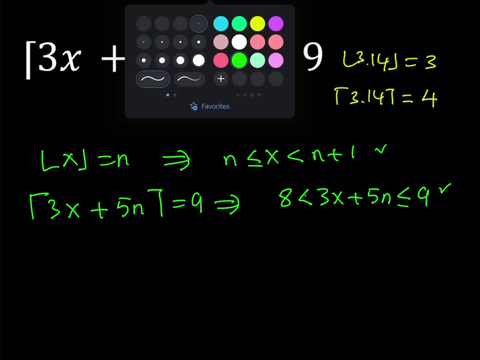 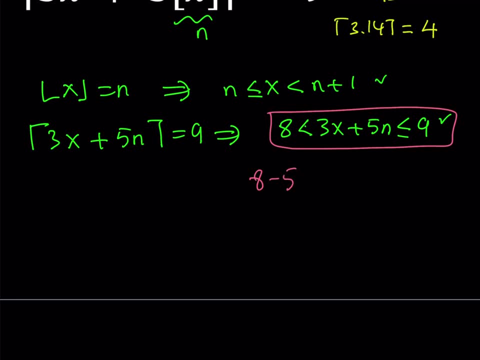 and this one, and this one. Let's go ahead and work each one. So I'm going to start with this one. Let me go ahead and simplify that First. if you subtract 5n, you should be getting this: Let's. 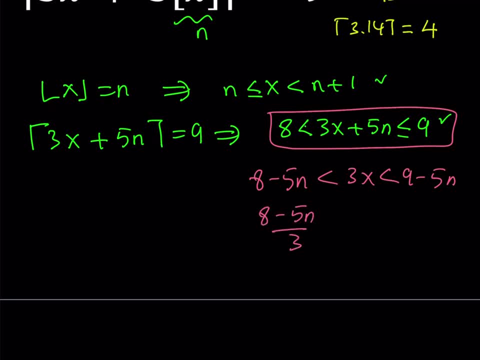 divide everything by 3. Because 3 is a positive quantity, so it would not matter, like the inequality would not change. All right, so that's one of my inequalities that I'd like to be using, and the second one comes from: 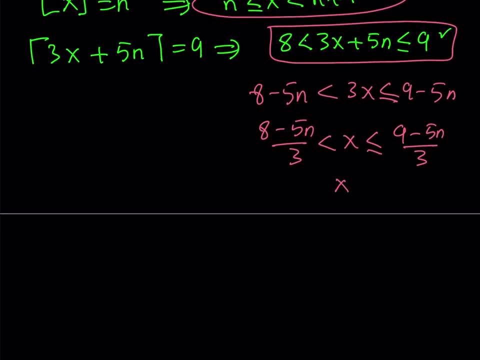 here. So let's go ahead and copy that here. x is between n and n plus 1.. So I do have two inequalities, So it's kind of like a system of inequalities. Let's go ahead and solve this system. Now we have two variables. 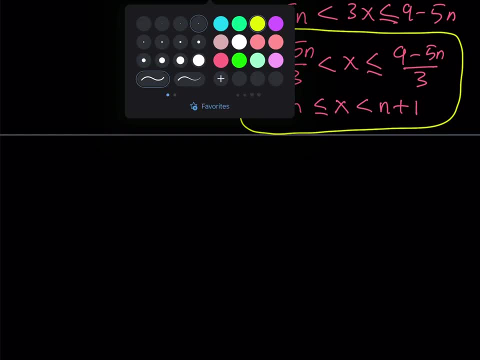 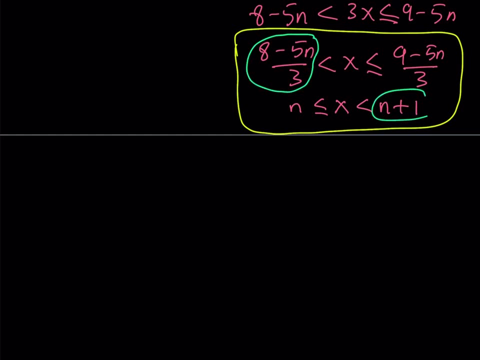 So, but we can work with the boundaries, So we do have a lower bound and an upper bound, So we can go ahead and compare them. For example, 8 minus 5n over 3 needs to be less than n plus 1, obviously. 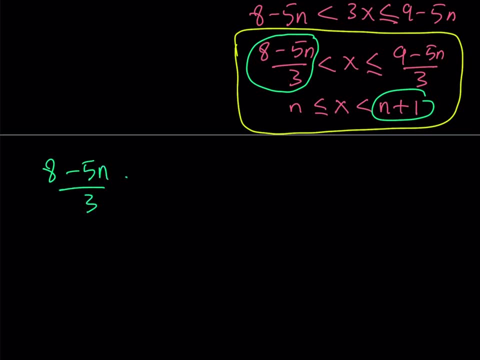 right, So let's go ahead and write that down as an inequality. 8 minus 5n over 3 needs to be less than n plus 1.. If you go ahead and multiply both sides by 3, you get the following, And I'm putting: 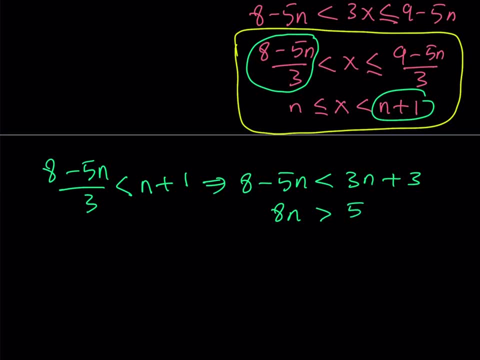 n's on the same side, 8n is greater than 5. And n is greater than 5 eighths. So that's one of the inequalities solved. Let's go ahead and solve the second one Now. in the second inequality, what I need to do is compare these two quantities. 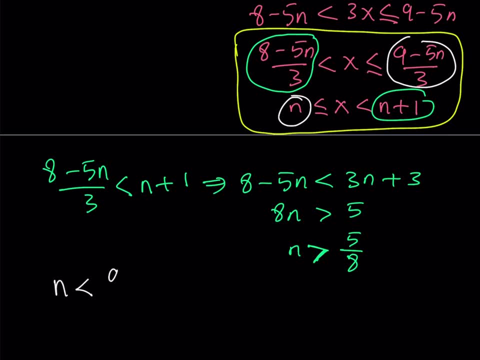 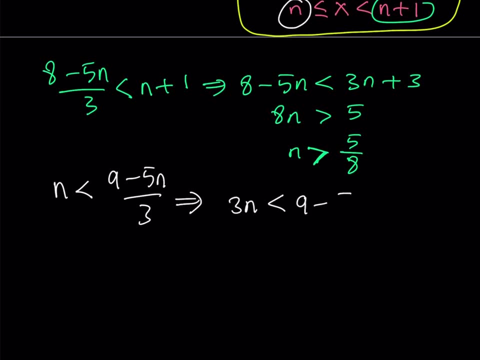 Obviously, this means that n is less than 9 minus 5n over 3. And this implies 3n is less than 9 minus 5n. If you put both numbers on the same side, you should be getting n is less than 9 over. 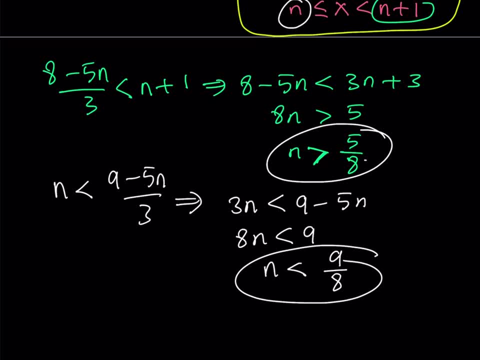 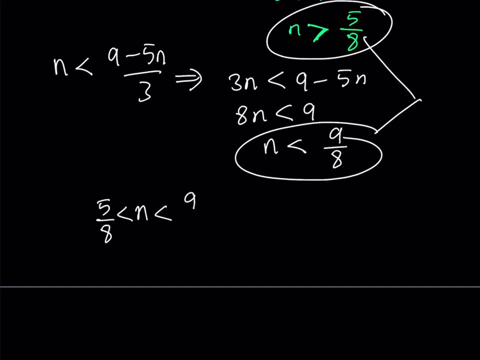 8.. So I got this and I got that, So I got to put these two together. That means that n needs to be between 5 over 8 and 9 over 8.. And remember that n is an integer, because the floor value or the 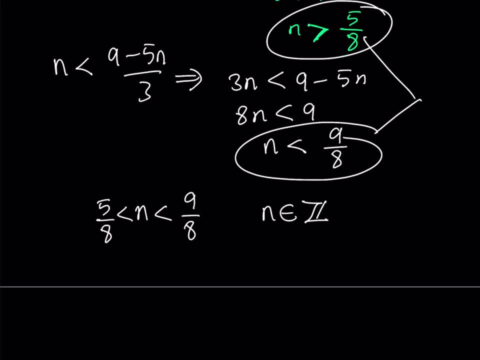 ceiling value, by definition of any quantity is always an integer. So the only integer that can go in this interval is n equals 8 over 8, which is 1.. So n needs to equal 1.. Great Now. having said that, now what I'm going to do is I'm going to go back here and substitute n equals 1 into both. 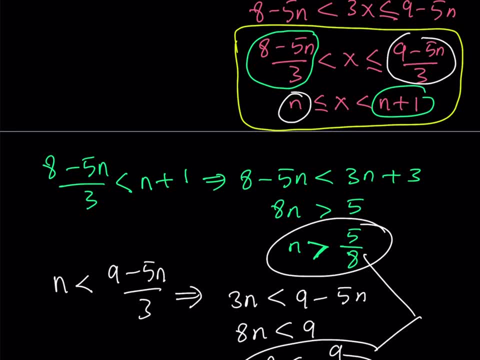 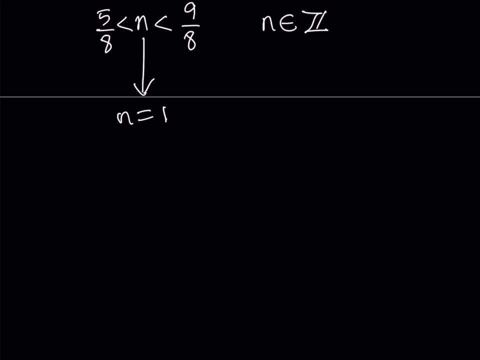 of these inequalities and get a system from there, And I'm going to solve that system And eventually, hopefully, we can turn that into an equation. So, like I said earlier, we're going to go back and forth between equations and inequalities. So let's go ahead and substitute n equals 1 into both of.